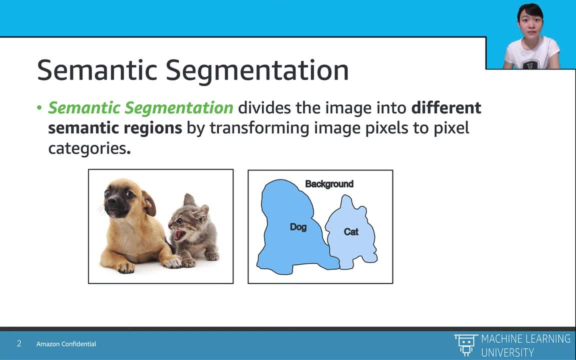 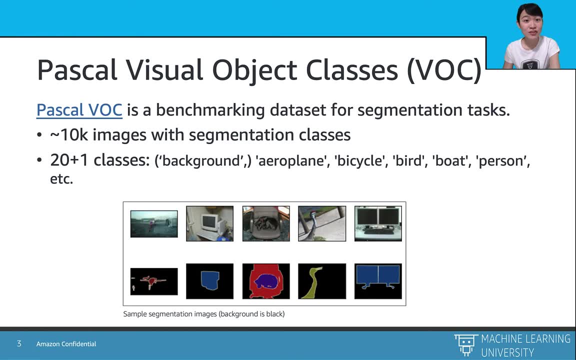 either dog, cat or background For benchmarking dataset for semantic segmentation tasks. we will introduce two most famous ones. The first is Pascal visual object classes dataset or SEMATIC-BASIC, which is focused on mass segmentation of images in terms of size, size. 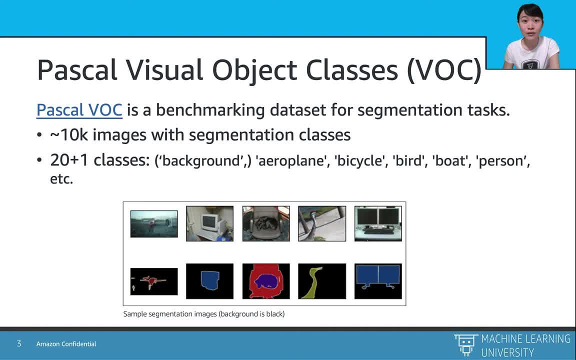 and properties, as well as the dog, cat and background. It contains around 10,000 images with 20 semantic classes, or 20 plus one if we add the background. in The semantic classes include bicycle, bird boat, bottle, bucket, car, cat, person and more. 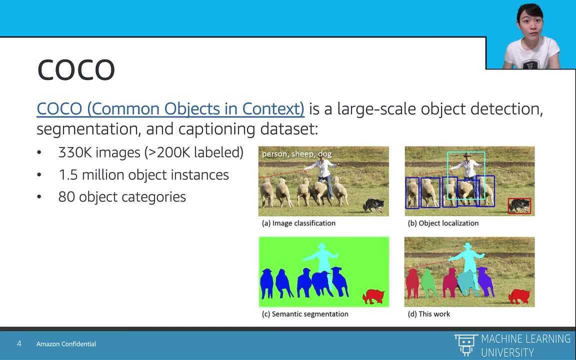 And then another famous benchmarking dataset, for not only semantic segmentation but also instance segmentation, is this microsoft coco dataset. so what is the difference between instance segmentation and the other tasks? if we look at the plot here, well, the previous object vaccination dataset focus on first the image classification or the object bounding boxes. 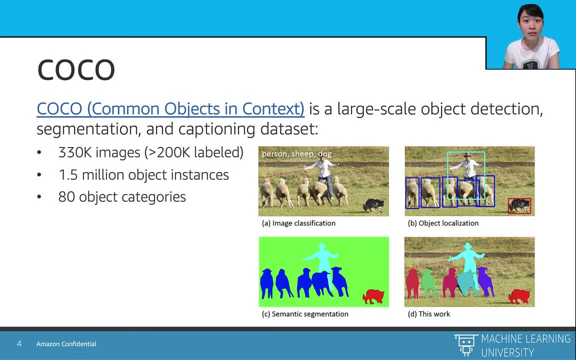 localization or semantic pixel level segmentation. the coco dataset focus on the semantic individual object instance, so coco is short for the common objects. in context, it introduces a large, rich anatole dataset comprised of images, this picking complex everyday things of common objects in their network natural contacts. so coco is a large scale data set with 330 000 images, where 200 000 of them 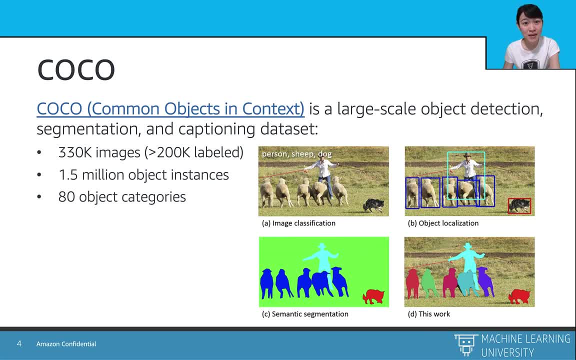 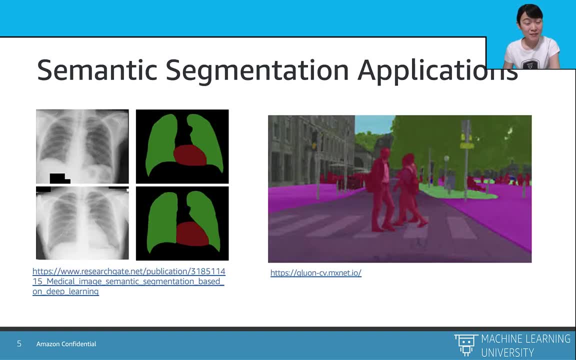 are labeled and there are 1.5 million object instance and 80 object categories in total. so semantic segmentation have a lot of applications on our left. it's an example of semantic segmentation in medical doping. it was a model on the japanese societies of radiology technology.